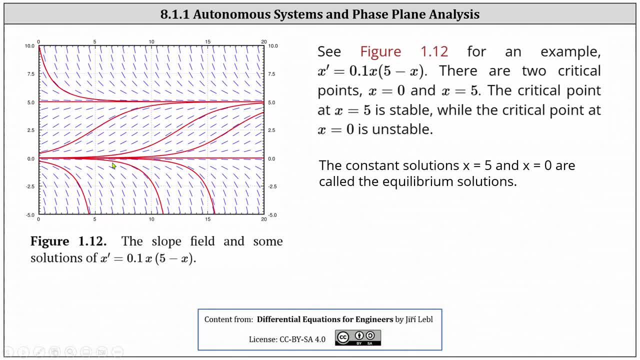 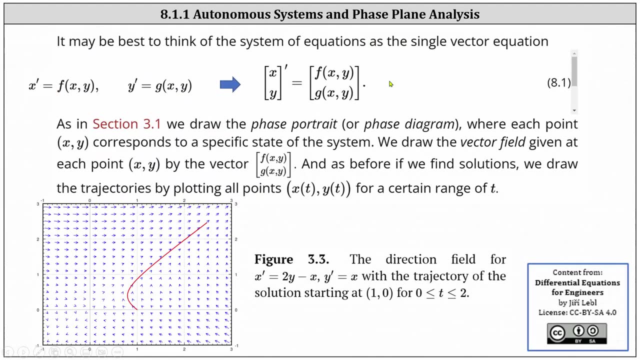 around x equals zero. as t approaches infinity, the solution no longer approaches: x equals zero. The constant solutions x equals five and x equals zero are called the equilibrium solutions. So now, going back to an autonomous system, it may be best to think of the system of equations. 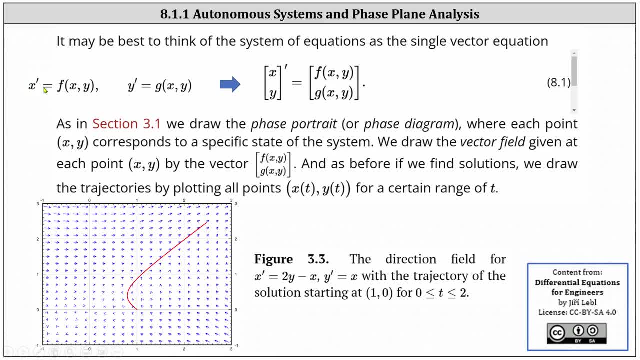 as a single vector equation where, if we're given x, prime equals f of x comma y and y prime equals g of x comma y, we can think of this as the derivative of the vector xy equals the vector f of x comma y, g of x comma y. 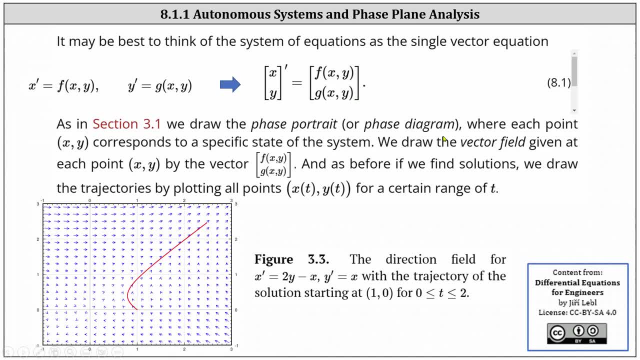 As in section 3.1, we draw the phase portrait or phase diagram where each point x comma y corresponds to a specific state of the system. We draw the vector field at each point x comma y by the vector given by f of x comma y, g of x comma y. 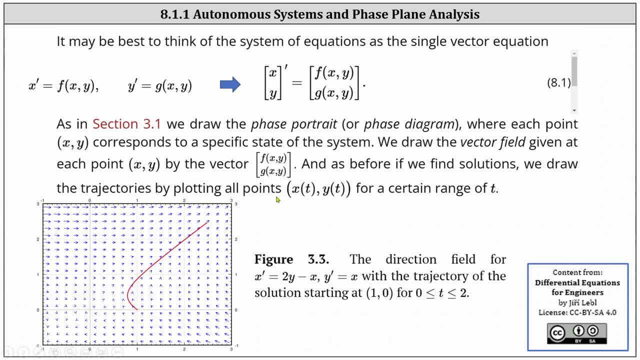 And as before, if we find solutions, we draw the trajectories by plotting the points x of t, comma y of t for a certain range of t. So below we have the direction field for x, prime equals two, y minus x and y prime equals x. 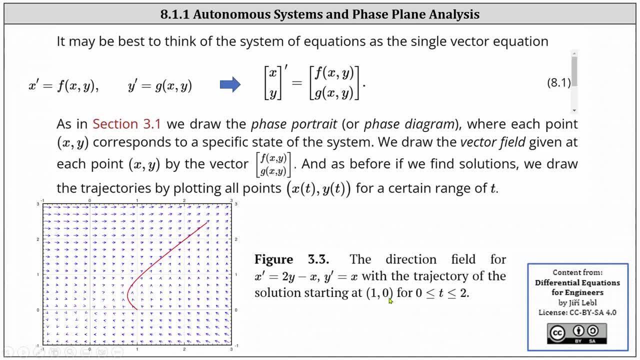 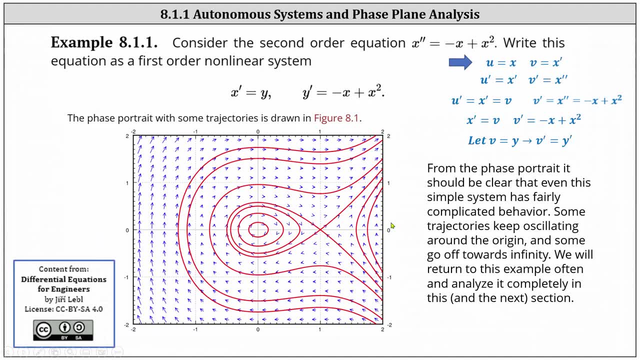 The trajectory of the solution, starting at the point one comma zero for t, over the closed interval from zero to two is graphed in red. And now let's consider an example. Let's consider the second-order equation: x double prime equals negative x plus x squared. 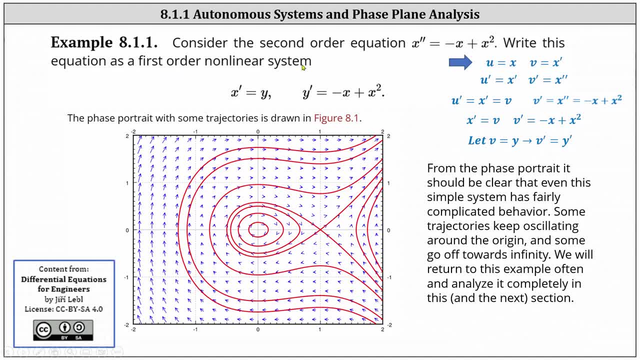 We're first asked to write the equation as a first-order nonlinear system which is given as: x prime equals y and y prime equals negative x plus x squared. Let's first talk about where this came from In general, to write a second-order equation. 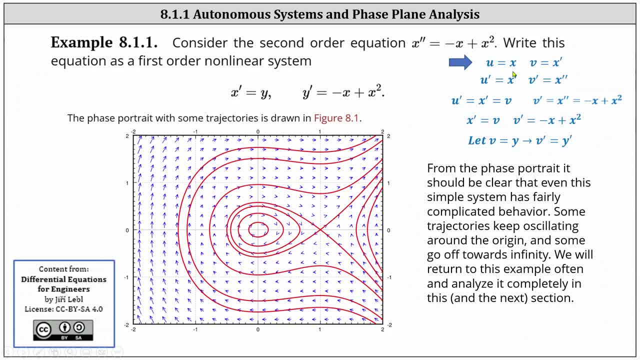 as a first-order system, we begin with u equals x and v equals x prime. From here, u prime equals x prime and v prime equals x double prime. Well, we know, x prime is equal to v, which gives us x prime equals v. 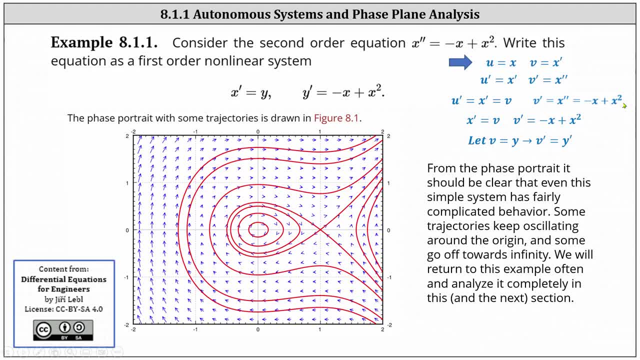 We know x double prime is equal to negative x plus x squared, which gives us v prime equals negative x plus x squared. So we could have written the first-order system in this form, but notice, our text is using y instead of v and therefore we simply replace v with y. 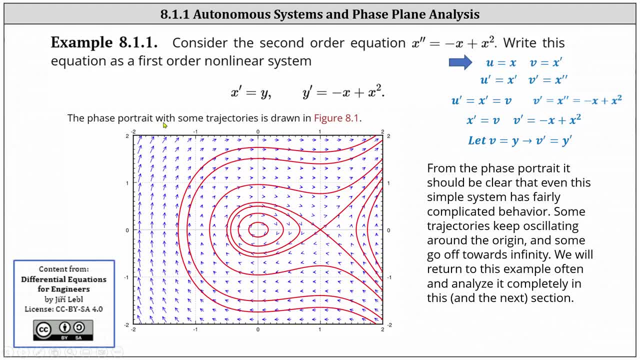 and v prime with y prime. The face portrait with some trajectories is drawn in the figure below for the first-order nonlinear system. From the face portrait it should be clear that even this simple system has fairly complicated behavior. Some trajectories keep oscillating around the origin. 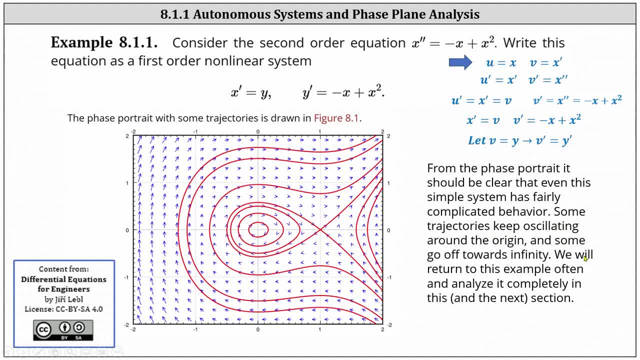 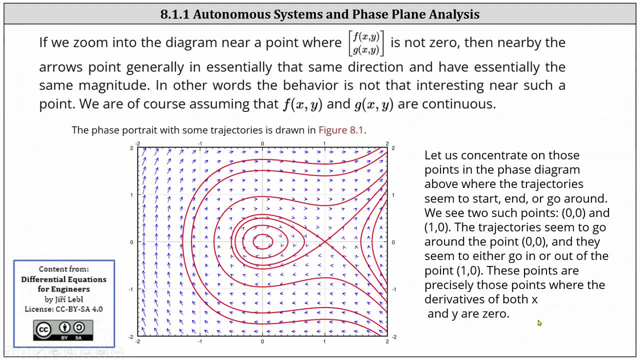 which we see in this region here and some go off towards infinity. We will return to this example often and analyze it completely in this and the next section. If we zoom in on the diagram near a point where the vector f of x comma y, g of x comma y is not zero, 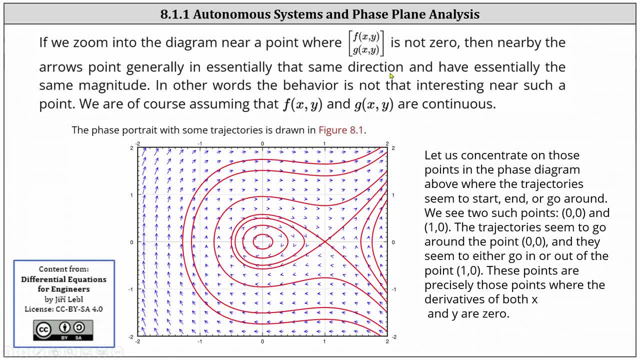 then nearby, the arrows point generally in essentially the same direction and have essentially the same magnitude. In other words, the behavior is not that interesting near such a point. We are of course assuming that f and g are continuous. Let us concentrate on those points in the phase diagram. 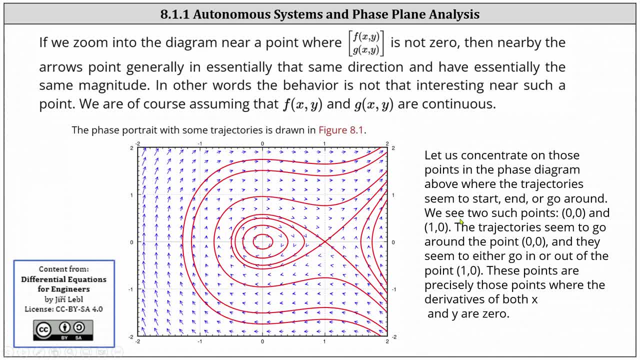 where the trajectories seem to start, end or go around. We see two such points: zero comma zero, which is here, and one comma zero, which is here. The trajectories seem to go around the point zero comma zero and they seem to either go in or out. 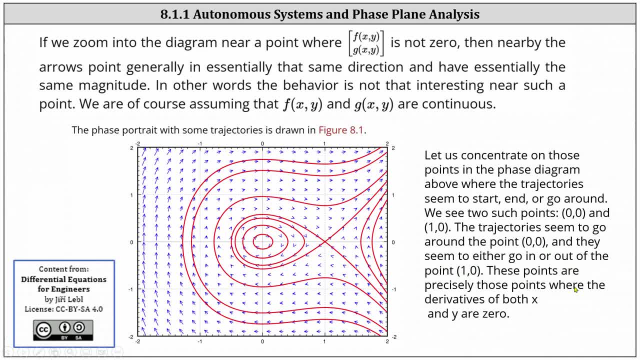 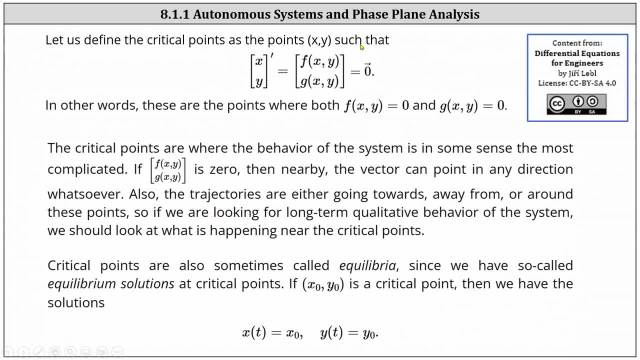 of the point one comma zero. These points are precisely those points where the derivatives of both x and y are zero, The critical points of the points x comma y, such that the derivative of the vector xy is equal to the vector f of x comma y, g of x comma y. 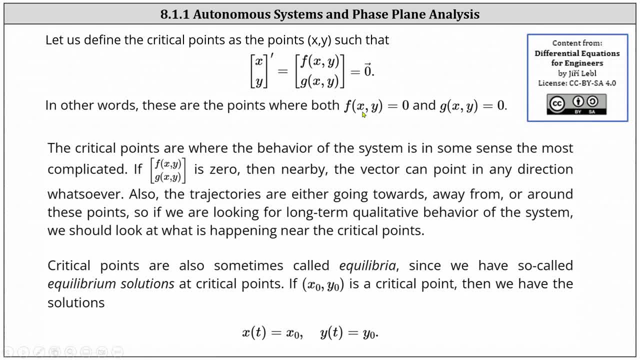 equals the zero vector. In other words, these are the points where both f of x comma y and g of x comma y equals zero. It's important to notice here: they both must be zero in order for x comma y to be a critical point. 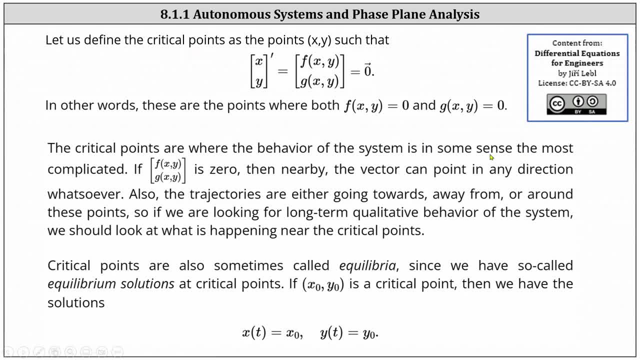 The critical points are where the behavior of the system is in some sense the most complicated. If the vector f of x comma y, g of x comma y is zero, then nearby the vector can point in any direction whatsoever. Also, the trajectories are either going towards away. 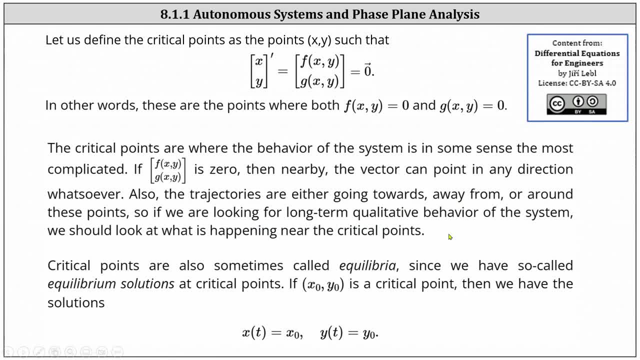 or around these points. So if we're looking for, let's say, a point, we're looking for long-term qualitative behavior of the system. we should look at what is happening near the critical points. Critical points are also sometimes called equilibria.